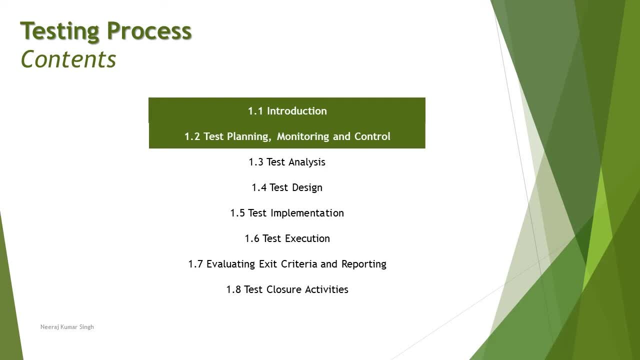 which you can see on the screen now, and, of course, we will be getting started with the introduction and test planning as a part of this tutorial and, of course, we will be talking a little bit in more detail and, of course, with the advanced approach of understanding how exactly to make. 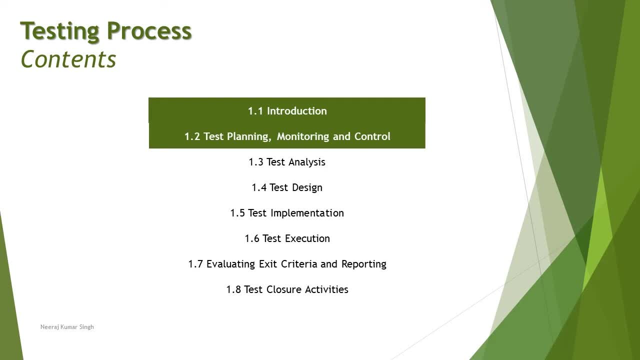 decisions at a certain point of time. So this entire syllabus will help you to determine what is the responsibility of the test manager at different point of time and different stages and different phases of the life cycle. So this tutorial will be slightly longer, because you need 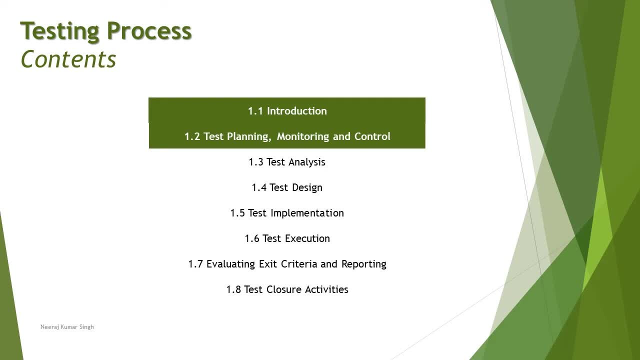 to understand a lot of things before you can actually look forward to write the examination. So be patient and learn everything in a detailed way. The very first tutorial today we are covering is, of course, the introduction and the first part of the 1.2, that is, test planning. and in the second, 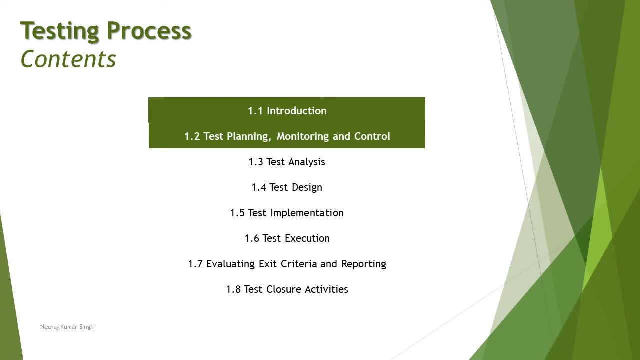 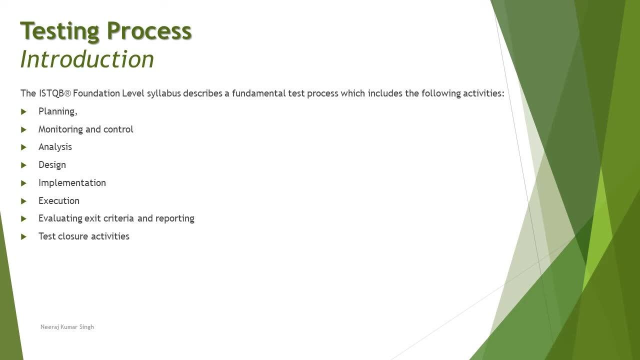 part of this tutorial, we will be covering the monitoring and control. Of course, from the beginning, we will be talking about the test process Now. initially, the test process discuss about the entire testing life cycle and talks about a lot of phases like planning, monitoring and control. 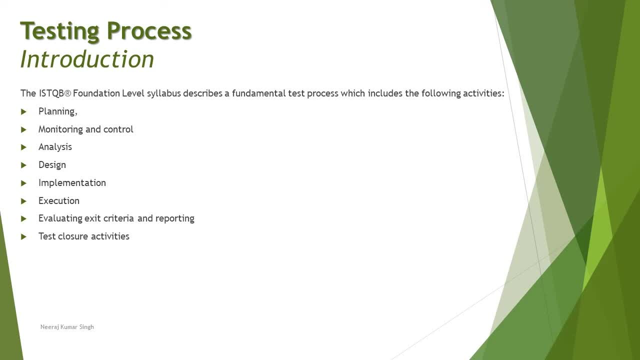 analysis, design, implementation, execution and evaluating exit criteria and reporting and, following that, the test closure activities. Now, each of these stages has several activities to be discussed and has major responsibility of the test manager in order to monitor, plan for all these activities and definitely take necessary control actions at different point of time. 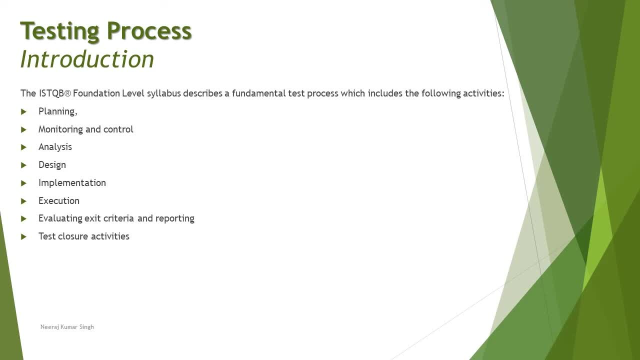 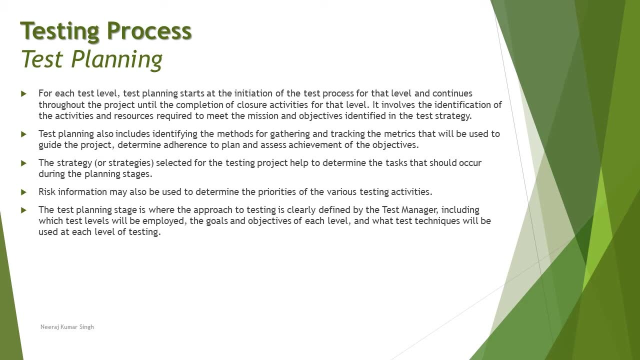 So let's look forward to what we have got in our syllabus from the test planning point of view. As a part of the test planning, first of all, planning is for the overall life cycle of testing, as well as the test levels which you may have within each of these phases. Now, of course, 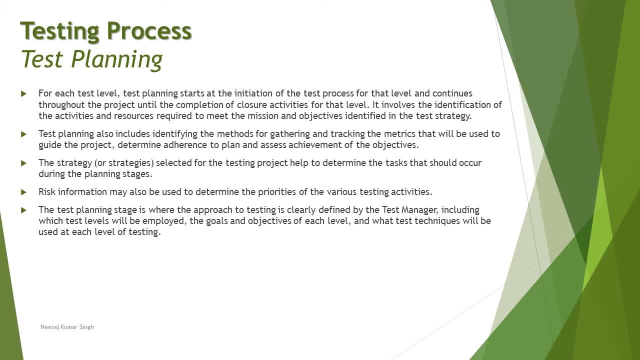 when we say the test levels, we are talking about unit integration system acceptance and a lot of other non-functional levels which are being conducted as a part of entire life cycle. So test planning is the major responsibility of the test manager, where test manager follows the project plan and schedule in order to determine. 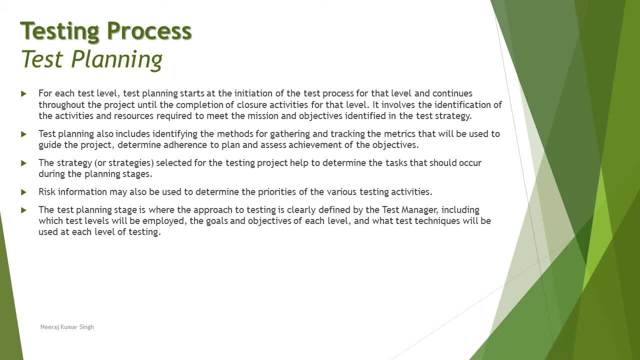 the overall plan of the life cycle and in fact the initial planning for the test levels can also be done right at the test planning phase itself, because you don't just wait for the stages or different levels to come into picture and start thinking of what to do there. So, test manager. 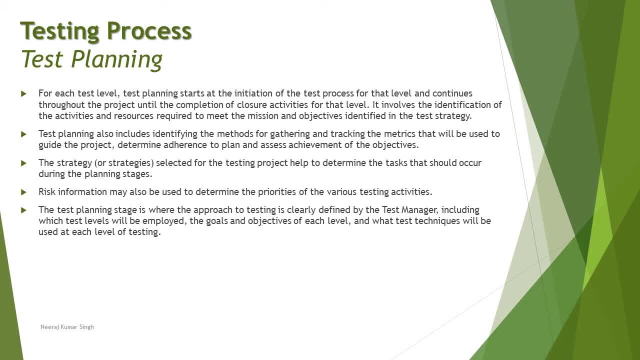 has to be well planned for any of the levels which you will be conducting as a part of the overall life cycle and, of course, the most important thing here is to plan in a early stages- is to align all these activities with those of the software development lifecycle. 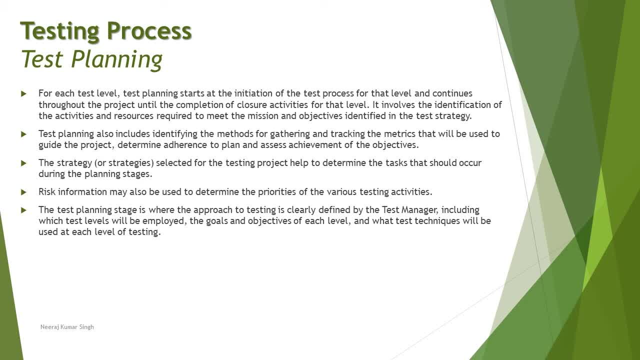 activities. I hope you remember from your foundation again that a good characteristics of testing involves a development activity with a corresponding testing activity. So, no matter what you do, all your activities must be aligned with those of the development activities, like architecture, design creations or development of the codes must all be, you know, aligned in such 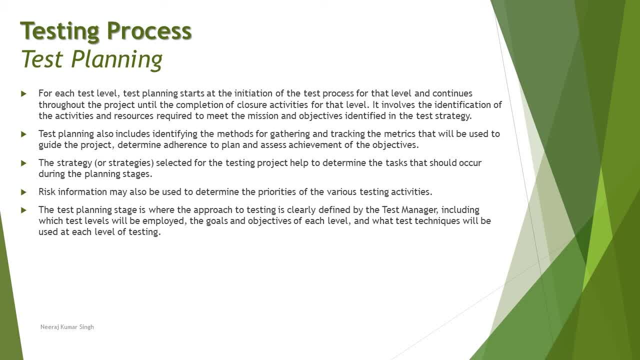 a way that, as soon as the code is available, you start with the unit testing, or as soon as the unit testing is done, simultaneously you can start with integration testing and a lot, many other things, including the entry and exit criteria of each level. talking about the availability of the code, 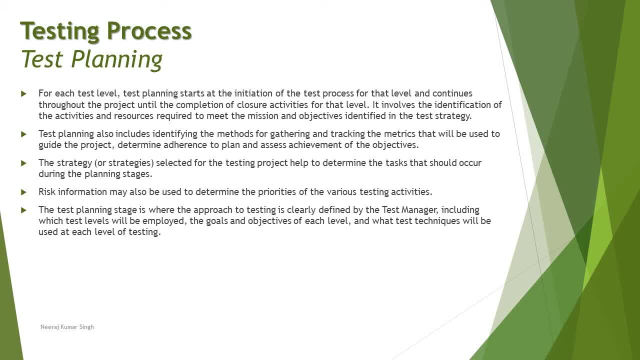 in order to begin with certain activities. So, yes, the planning definitely plays a vital role, and test planning also includes identifying the methods for gathering and tracking the matrices. We do remember from the foundation that one of the activity of the test planning phase is to select the matrices. Now, here, being a test manager, you 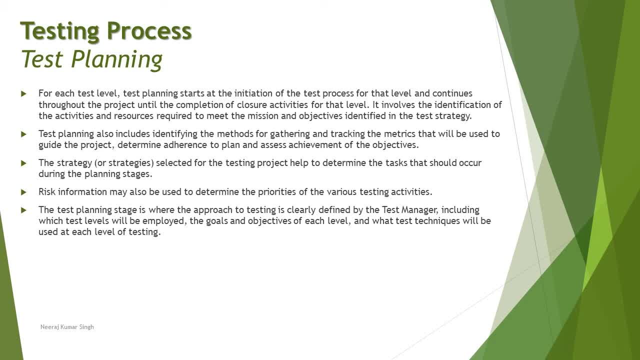 will be collecting different matrices in order to determine that what matrices will be helpful at different point of time during the entire lifecycle and how they will help you to monitor the progress on the project. and definitely, these matrices will only be the thing which will help you to determine if any control actions are necessary at any point of time to be deployed. 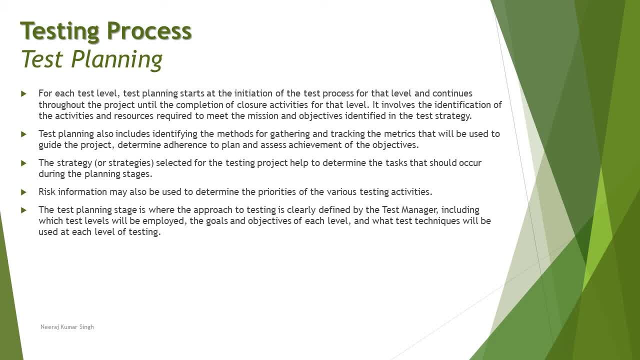 The strategy also plays a vital role here, which is definitely selected well before the test planning and definitely there are several approaches which you can collectively call it as a strategy, and we will be talking about them in more detail in upcoming chapters. so don't worry about that, and the strategy selected for the testing project will 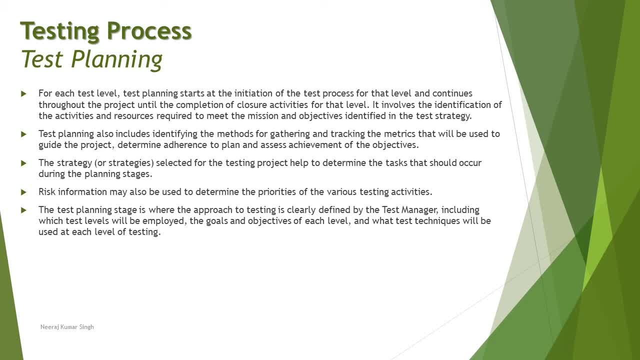 definitely help you to determine the task- and that should occur during the different planning stages- and, of course, how exactly your effort will be allocated for each and every activity in order to accomplish the goal of the test. So, yes, this is a strategy that we will be talking about in. 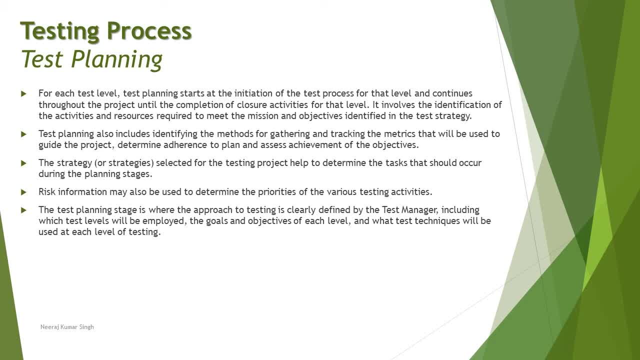 testing and achieve the objective of testing. also, to add, we have risk analysis being conducted at any point of time, so if you are following a risk-based approach, the risk information will also be used to determine the priorities of various testing activities. sometimes, a lot of certain activities will be pre-pwned in order to meet the expectations or mitigate the risk, which 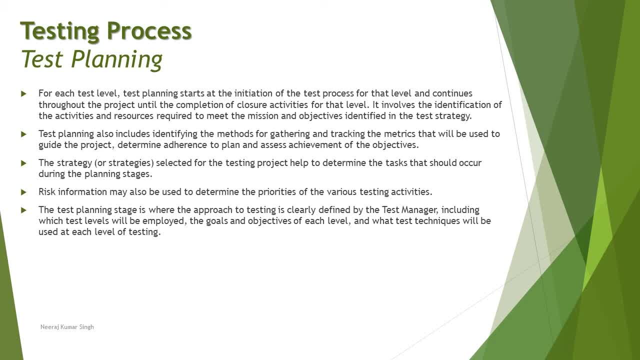 you would have identified and test manager. being a test manager, you have to keep account of all the project risk items as well, because you don't want anything to hamper your schedules and deliveries at any point of time. the test planning stage is also where the approach of to testing is clearly. 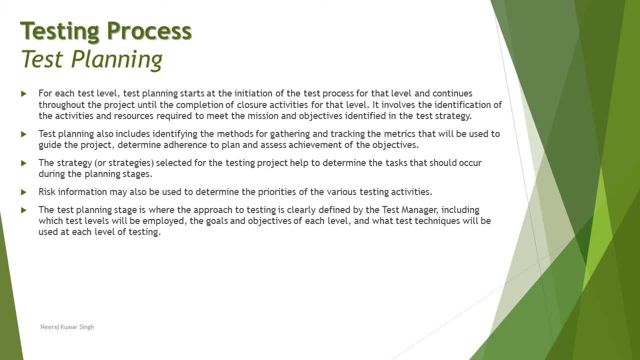 defined by the test manager, including which test level will be employed, the goals, the objective of each test level and what techniques will be used at each level of testing. so, right from the planning phase, you determine everything like what levels we will be conducting, how we will be organizing them. 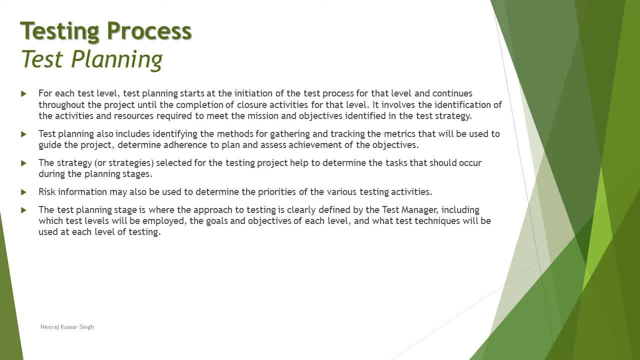 what kind of tools do we have to support? and and, and of course, we are talking about the techniques, like you know, equivalence partition or you know decision table testing or any kind of. you know other techniques like mcdc or you know mcd, which is for non-functional testing. so, yes, test manager will be completely responsible for. 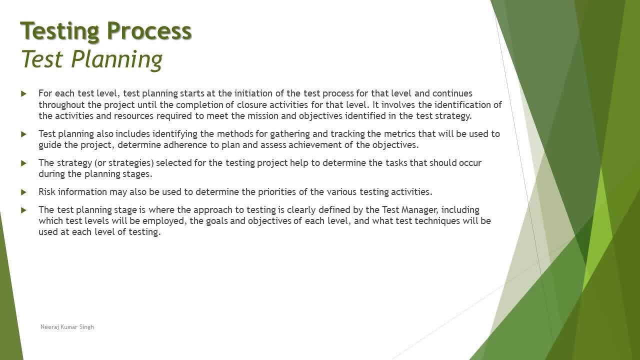 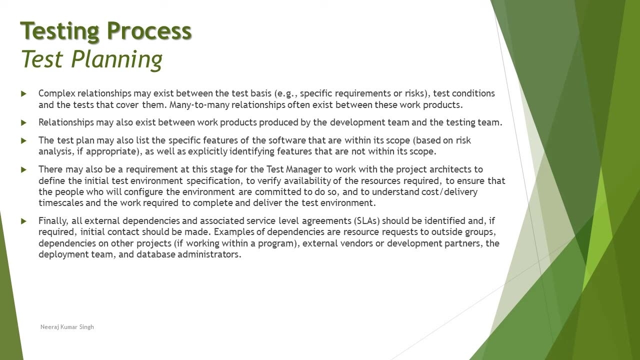 determining and selecting certain test techniques which will be best applicable to your process at any point of time to you know. make sure that you have a good success rate at the end of the day. further, to continue, we are talking about the traceability and relationships which may exist between the test basis and the test conditions. 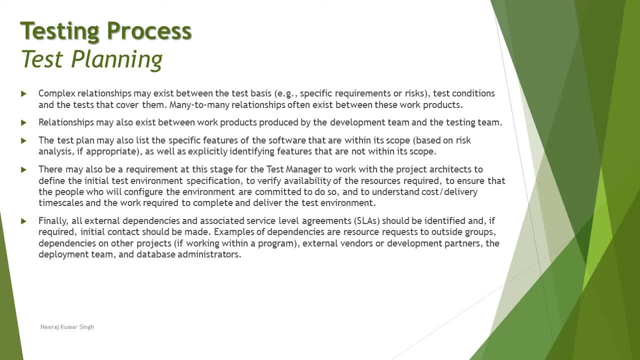 or the test cases which you are preparing. so again, being a test manager, it is your core responsibility to establish a good traceability option which allows different work items or work products to be integrated with each other. now we are talking about the integration between the test basis and the test conditions. of course, the test conditions are. 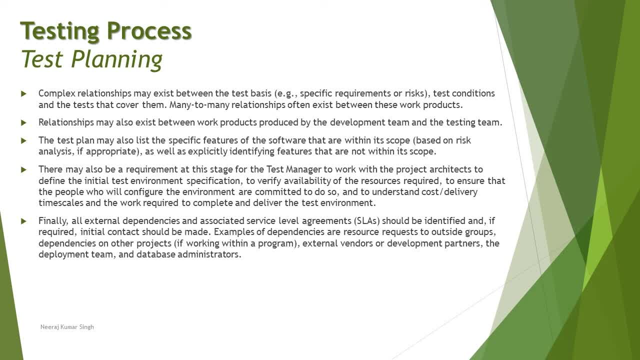 derived from a lot of specifications or designs or probably, sometime, even code. so the traceability must be established in order to see any kind of impact of changes on the test basis. So what if your two requirements are modified tomorrow? If requirements are being updated, then of course the 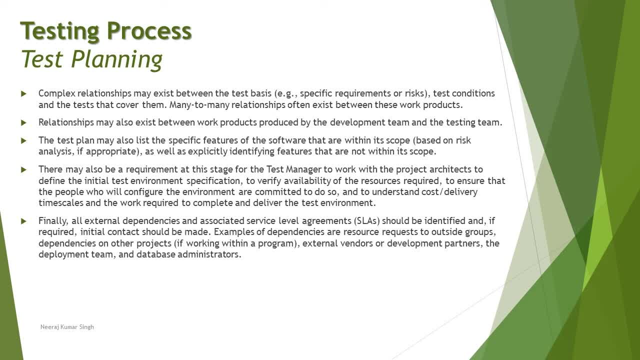 test cases might not be sufficient enough to fulfill the needs of the requirements at that point of time. So if, in case tomorrow, requirement has been modified and you have a good traceability between the requirement and the test cases which you have written for them, then of course this: 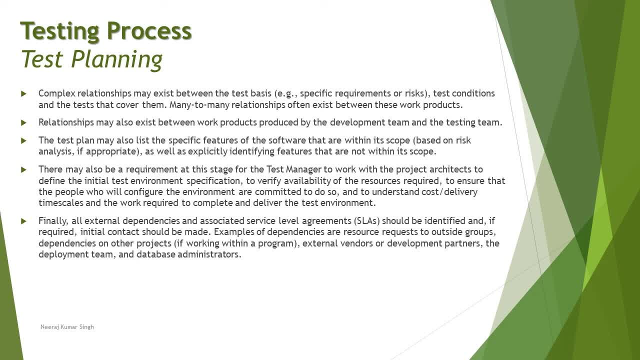 traceability will help you determine that. is your test cases still beneficial to achieve the complete coverage or you need to write something more in order to achieve the change as a part of the requirement changes? So, yes, building up and setting up a good traceability option could be as 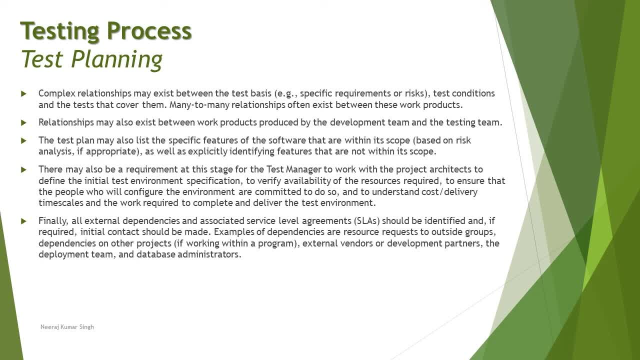 a part of the test management tool within your organization is definitely a responsibility of the test manager. Now, relationship is just not limited to the test basis and the test condition which you create. It could be even between the work products which are simultaneously created by different organizations or different team within your 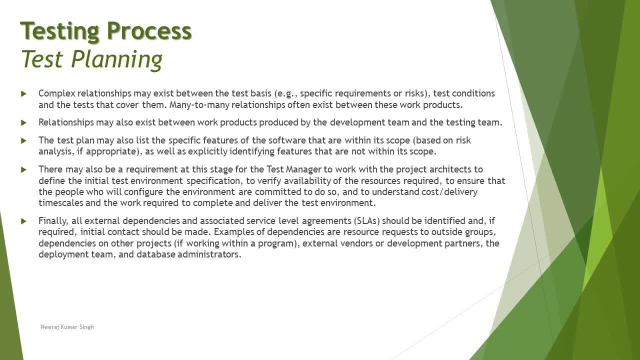 organization. For example, the design team creates a lot of artifacts, the development team create a lot of codes and algorithms and you know many other factors which might be integrated further with your executions or test cases. So you need to make sure that what are those work products? 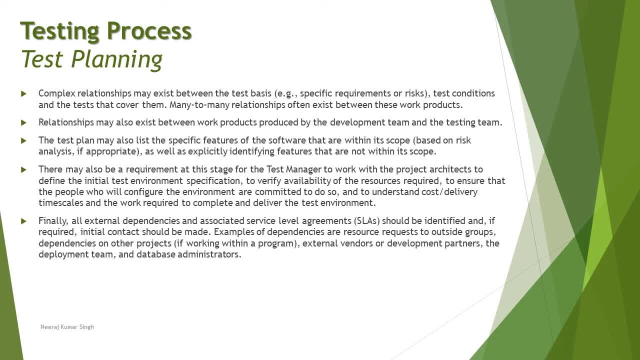 which you will be accessing to and will be having a traceability to. So make sure that if there is any kind of dependency, then you establish that in order to meet the requirements of the test. Further to the test plan, this will also have list of specific features of the software that are: 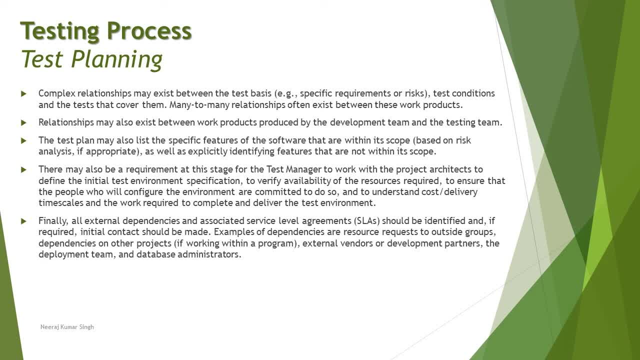 within our scope. So as a part of planning, you will determine what kind of you know part of the application you will be considering as a part of your testing scope, because not everything as a part of an application or release will be under the scope of testing. So when you determine the 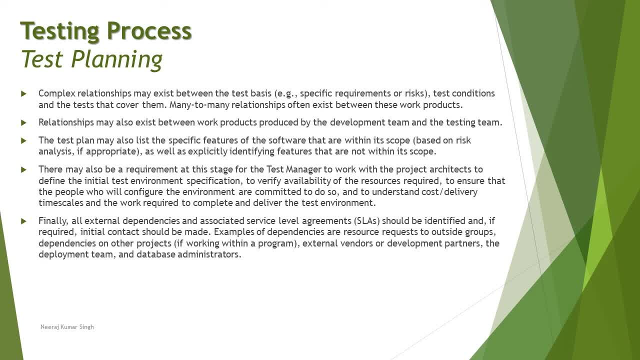 scope of testing. you do consider what part of the application will be under testing. what kind of features do we have to test? For example, you are considering the scope of testing of the application, the security parameters. you're considering the performance parameters, but maybe you're not. 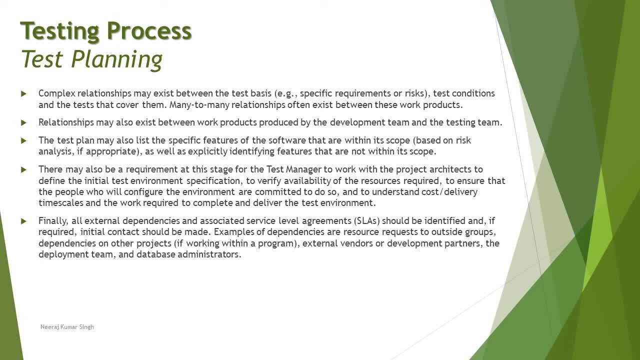 considering the portability feature this time, because this application is only supposed to work on one platform and it's not going to go into multiple platforms, so portability testing is not in our scope. so, of course, based on the requirement features and certain set of functionalities, you will determine what levels will be required. now there are also requirements. 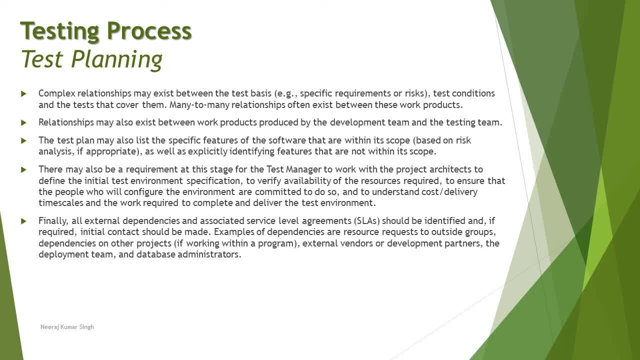 at this stage of the test manager to work with project architects to define the initial test environment specification. we do remember that deciding on what environment will be used will be a part of test analysis, because once you analyze all the requirements you can determine what environment will be sufficient for that. but initial establishment or, you know, selection, or 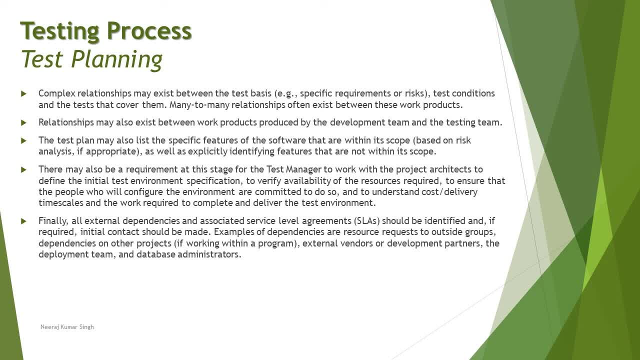 designing of the test environment can happen right at the test planning phase, because during test planning you can consult with the architects to see what kind of interface or what kind of architecture is the application going to have and based on that we can at least start laying down the foundation of the environment which will be. 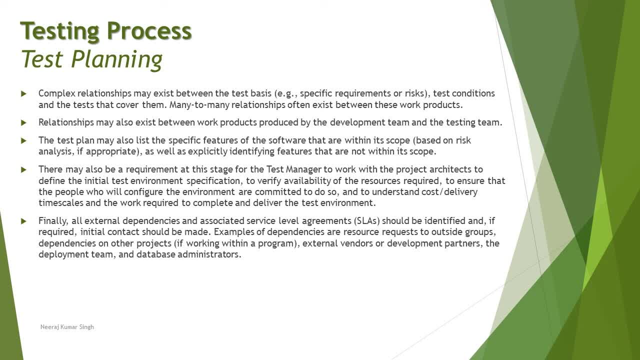 required to set up in future in order to run your test cases. so, yes, you can definitely, being a test manager, coordinate with the project architects to understand what is the tool or what is the software all about: what kind of platforms, what kind of architecture, what kind of web services. 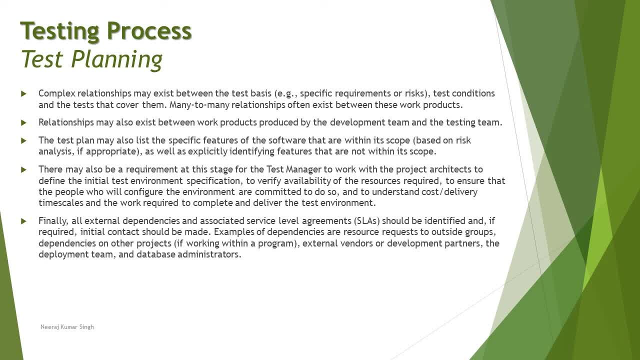 it is going to use, so you can start thinking about setting up your environment at that point of time. and, of course, at the same time, for all these activities you need to make sure what kind of time, what kind of effort, what set of you know, infrastructure and 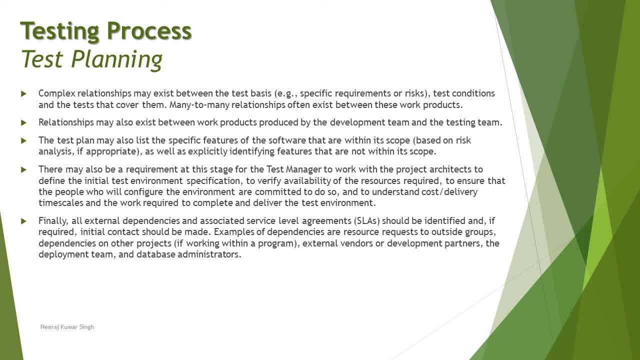 budget is required to conduct all these activities. so budget allocation will also be a part of planning phase itself. of course you will have something more to understand in detail this test estimation but yeah, from certain extent you do have some of the effort allocation and budget allocation right from the planning phase itself. finally, all external dependencies and associated 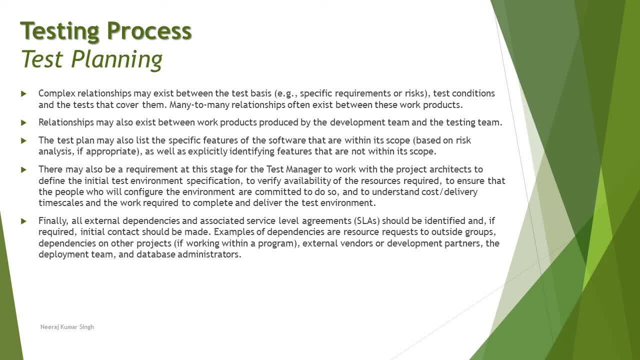 service level agreement should be identified and, if required, you can start planning your test at the initial. contact should be made. examples of dependencies are resources request to outside groups, dependencies on other project and external vendors of development partners, the development develop deployment team and the database administrators. so there are a lot of things.